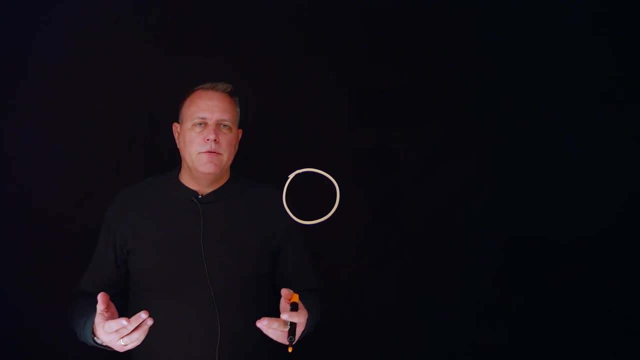 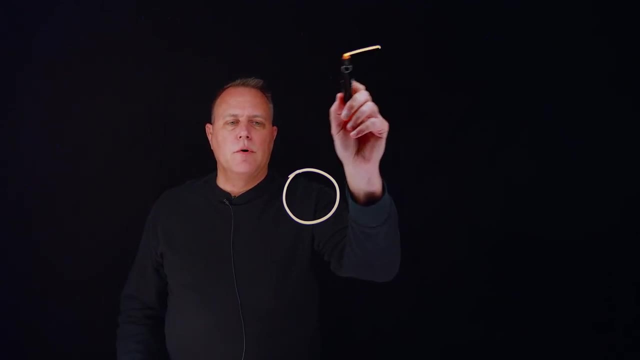 where is that object? what orbit is it in, so we can then try to figure out where it's going to be in the future. So an orbit, pretty straightforward. we'll make it simple. we'll call it some sort of an ellipse or circle or whatever shape it may be in as the object. 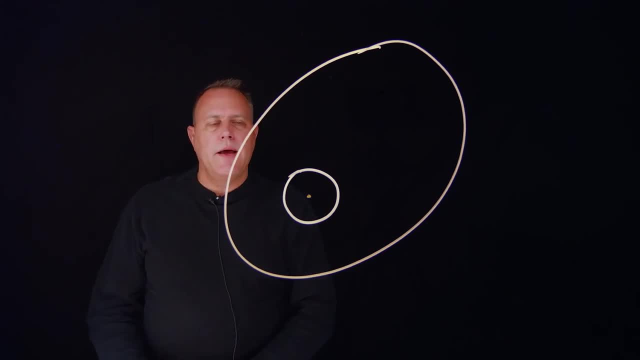 goes around the Earth. Now the problem is, I don't know that this is actually the shape of this object. So if I'm sitting on the Earth and I've got my little antenna here and I'm trying to collect some sort of data or signals from this object to try to figure out what 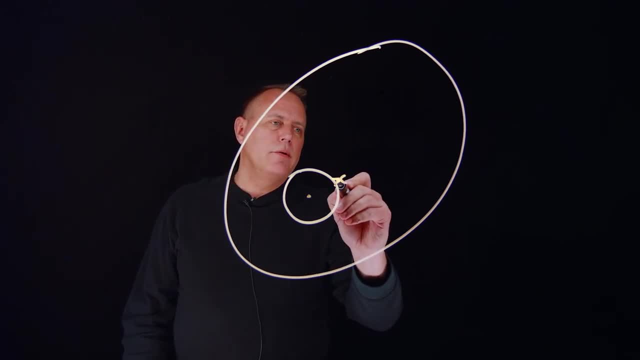 orbit it's in And that's a case where I might want to take a measurement. and if I can take a measurement, Let's say it's azimuth, elevation and range. it gives me a vector from where I am to where this object is that I saw. Let's imagine I'm a radar And I know where my sensor, my tracking, 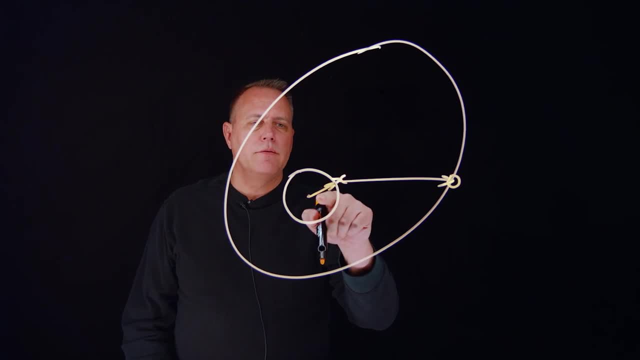 station is on the Earth, which means I know this vector. So if I know where the station is and I measure the direction and distance to the satellite, I know where it is at some point in time. We'll call this T1.. Now what I want to keep doing is I want to collect. 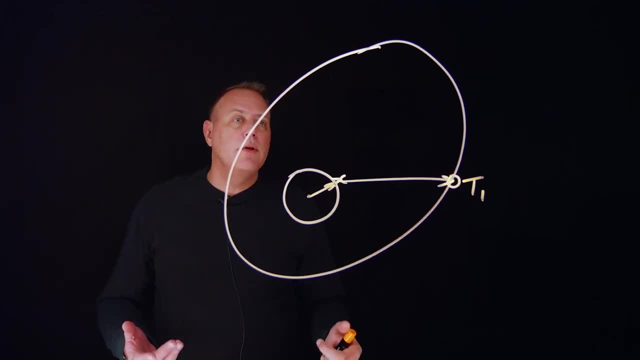 more data, because if I just only have one measurement, I don't really know anything other than there was a thing here at that time. So next, what I want to do is try to get another data point. So now what I'll do is I'll wait a little bit and let's say the. 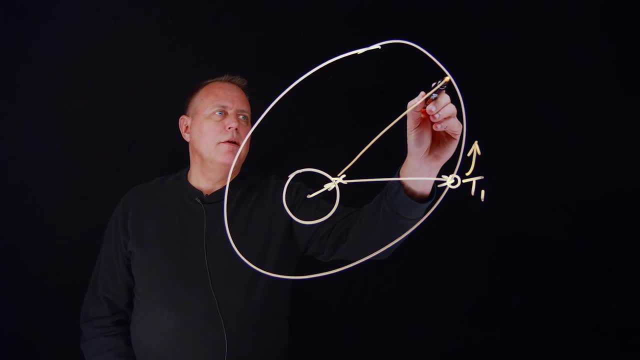 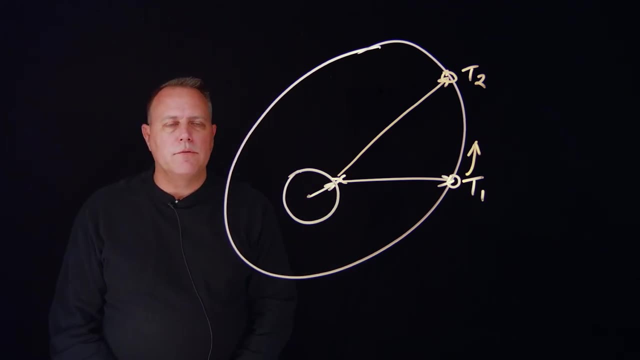 satellite's going in this direction And if I can get another measurement over here at time. T2, I now have two locations for the spacecraft Looking good so far And you can continue this process a little bit longer And maybe I get another measurement over here at time. T3. 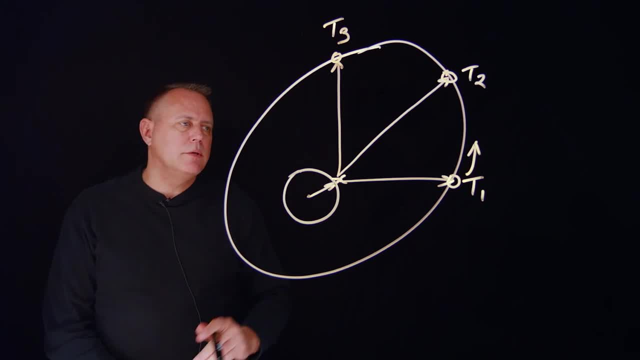 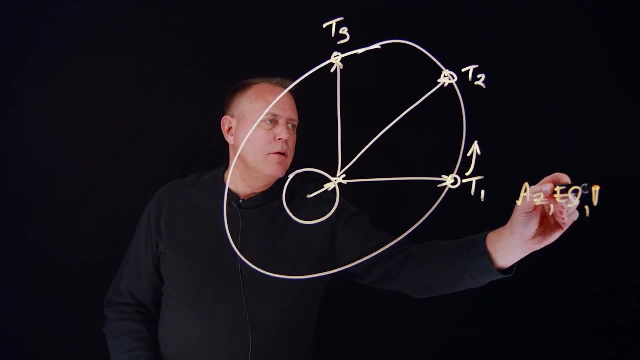 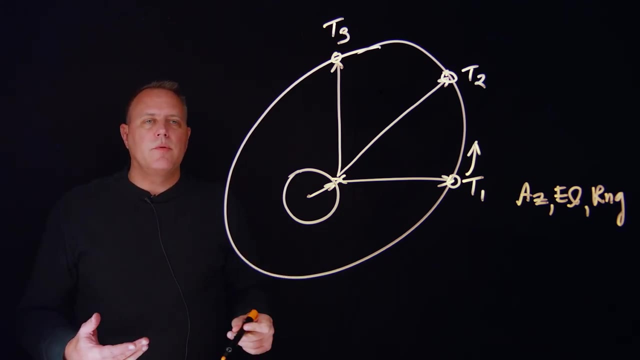 So now I have essentially three measurements, or three sets of measurements. So let's say, each set of measurements was azimuth, elevation and range. And in order to figure out the orbit of my spacecraft, what I really need to do is come up with what we call the state.